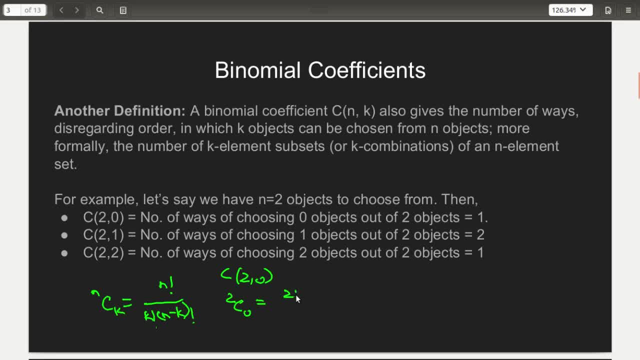 it as 2, c, 0, and I'll put in the values of n and k. I get 2 factorial upon 0 factorial into 2 factorial and this becomes 1, and that is what we saw earlier as well. so now that we know these two definitions, we can move on to our problem statement. so problem statement. 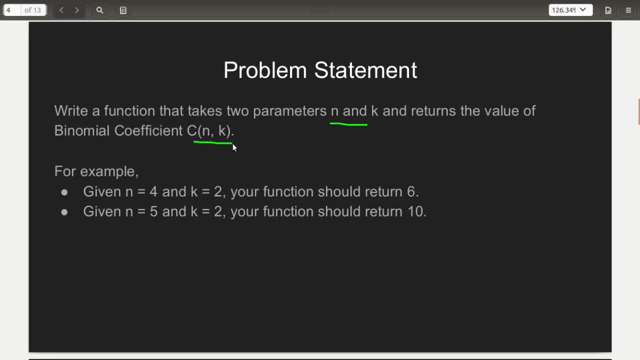 is very simple. it says: given n and k, calculate C n comma k. so for example, if we have n is equal to 4, k is equal to 1.. 2, we should return 6 and so on. so we just saw two ways to calculate C? n comma k. now 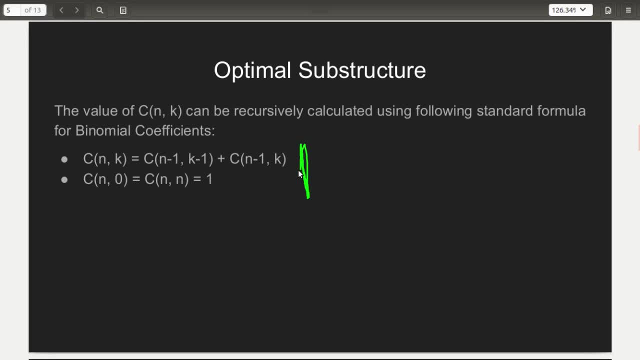 here is another standard formula. this also comes from combinatorics. so we have this recursive formula. what it does is it splits C n comma k into two parts: C? n minus 1 comma k minus 1 plus C n minus 1 comma k. so, in order to calculate, we split it into two parts and we 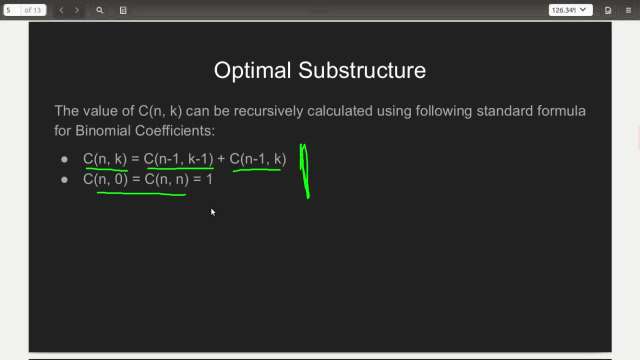 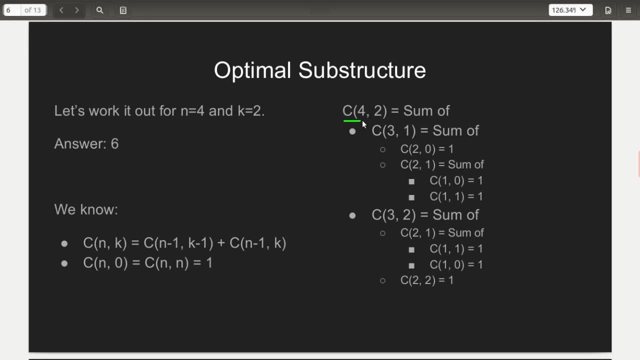 keep on splitting until we reach one of these base conditions. so let's work it out, for n is equal to 4 and k is equal to 2, so we have to calculate C 4 comma 2, we split it into two parts and we keep on doing until we reach the base conditions. 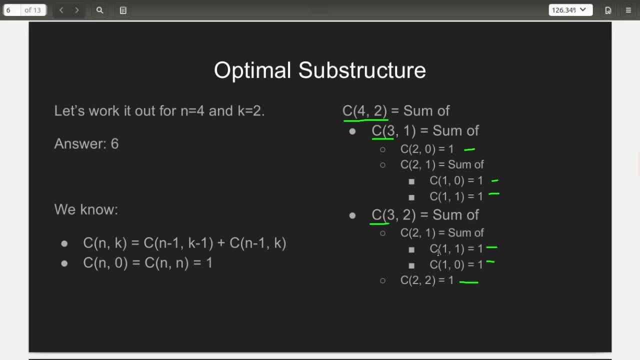 and once we reach at the base condition, we start substituting, substituting the values. so we add these two values to get 2 over here, and then we add these two values to get 3 over here. similarly, we add these two values to get 2, and we add these two to get 3, and finally, 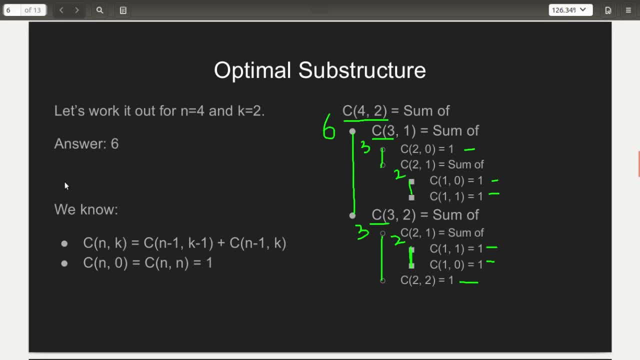 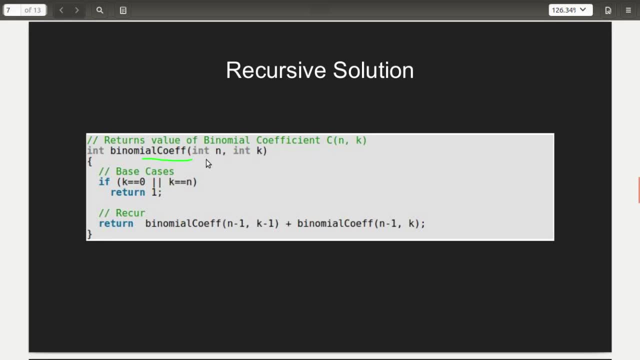 we add these two values to get 6, which is the answer. so let's see how to do this in C language. we have our method, binomial coefficient, that is, receiving these two parameters, and the base cases are what we just saw earlier. if k is equal to 0 or n, we return 1, if not, we simply split the problem into the two sub. 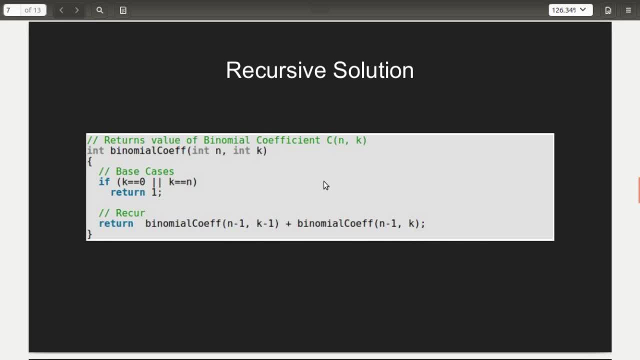 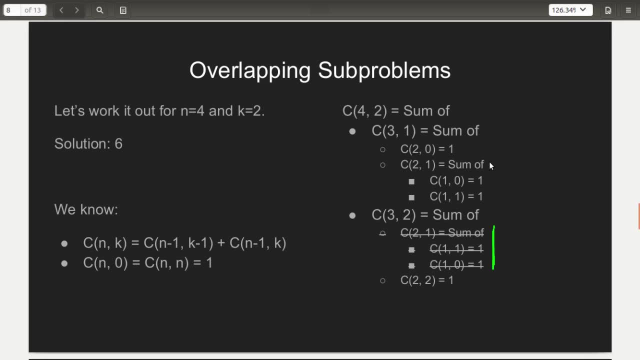 problems and we return the sum. so, if you notice, we actually recalculated C 2 comma 1 twice when calculating C 4 comma 2, so this problem has the overlapping subproblem property as well. because we are recomputing the, we are trying to solve the same problem multiple times. 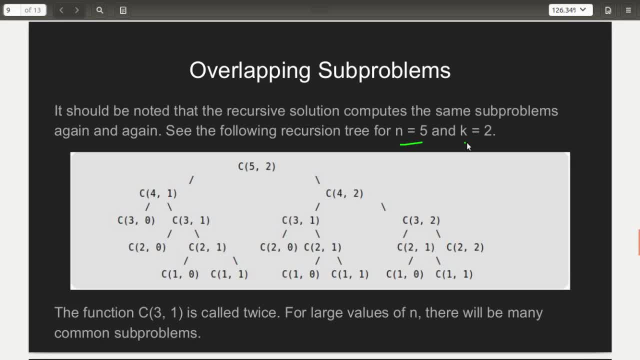 in fact, let us look at this another example, for n is equal to 5 and k is equal to 2. we have the recursive tree drawn over here and, as you can see, this whole sub-tree C 3 comma 1, is repeated over here and furthermore, 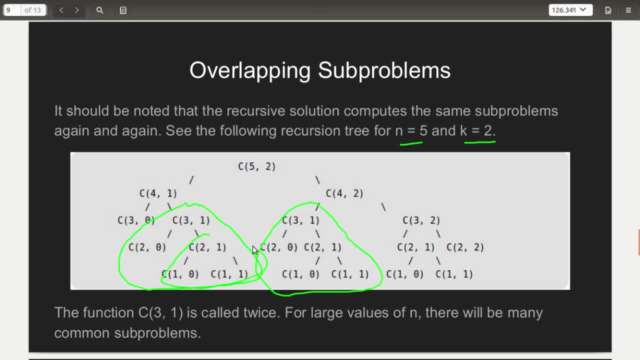 inside this sub tree we have this part C 2, comma 1, which is repeated over here as well as over here. so we see that we are solving the same problems again and again. and as the values of n and k increase, the size of this recursive tree will also increase and the 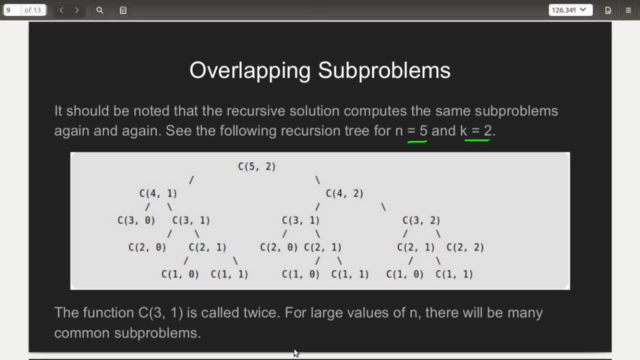 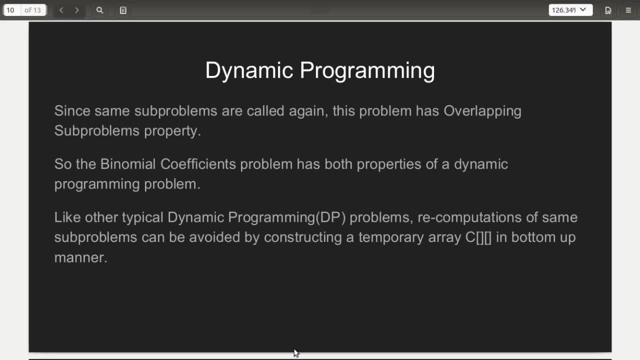 number of conditionals will also increase that we are redoing will also increase. so so we saw that this problem has the overlapping subproblem property and it also has the optimal substructure property that we saw earlier. so this classifies as a dynamic programming problem, and we know that when approaching dynamic programming problems, 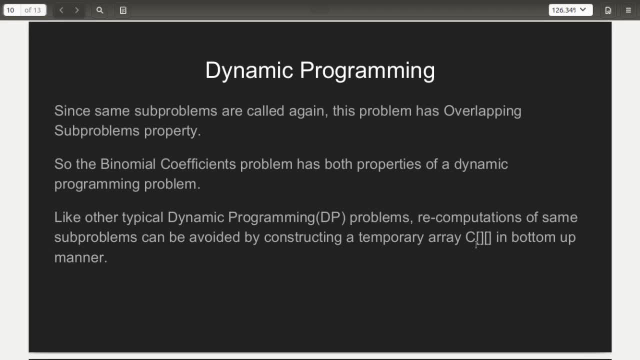 we can, instead of recomputing the same values again and again, sorry, instead of solving the same problems again and again, we can store the previously computed values in an array and use them whenever those are needed in the future. so let's see how this is done using C language. so we again have the same 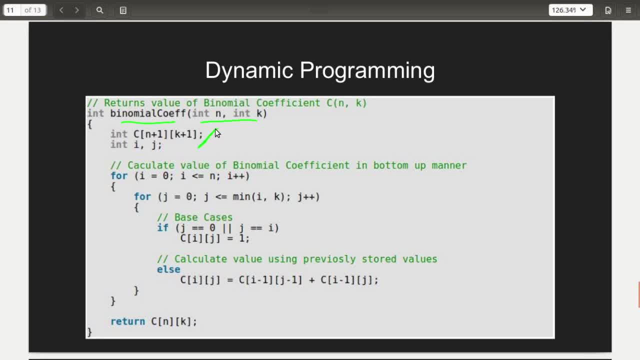 method over here with the two parameters. so we begin with creating a two dimensional table in which we will put into values and we run two loops. the first loop, done from I, is equal to 0 to n, and the second loop runs from j is equal to 0 to sinn, is our order alone again. so when we consider now inaretil, 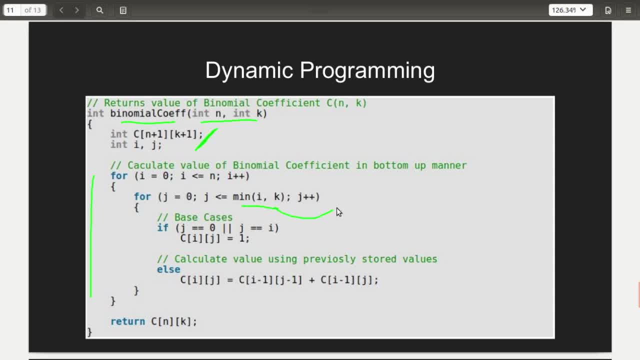 equal to n, and the second loop runs from j, equal to 1 to n for say Na, and so we solve Pr tak um. we need also to find out the type parameter, like in the form of min of i comma k. we'll get to this in a minute. so inside this loop, again we see that we are. 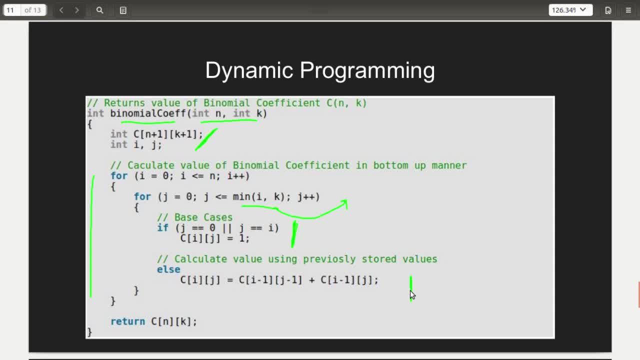 using the same formula, except this time we are not making recursive calls. so what happens here is again. we are looking for the base cases. if j is equal to 0 or i, we put in c i, j is equal to 1. however, if it isn't, instead of recursively calling the same function again. 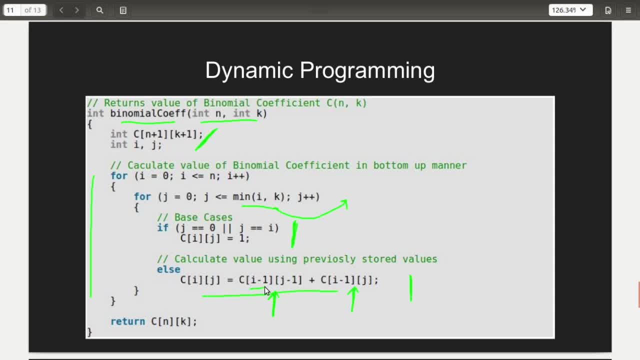 we are actually looking up in the table and using the values that were previously computed. so this is how we construct the table: c i comma j and finally, once our loops exit, we return the value of c n comma k. now why do we have this min i comma k over here? so if 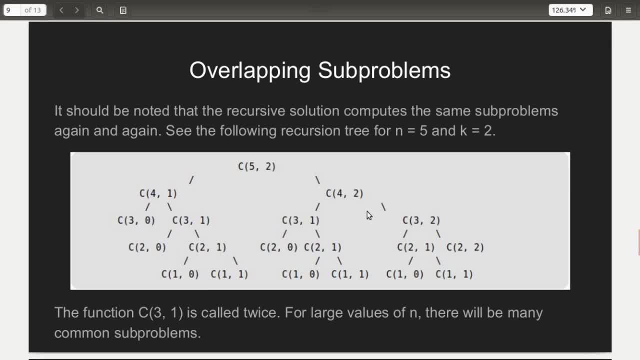 you remember- sorry, if you noticed- when we were calculating c four comma two, so we divided this into two parts. so, if you notice, when we were calculating c four comma two, so we divided this into two parts. so, if you notice, when we were calculating c four comma two. 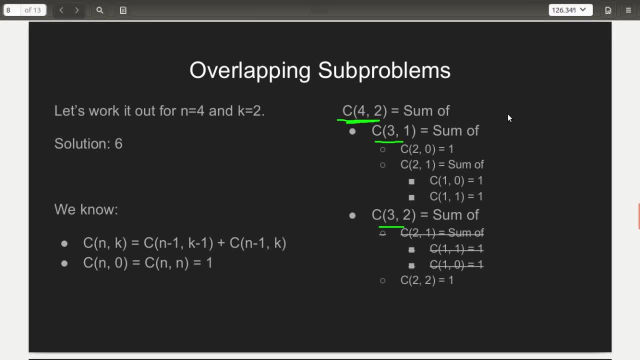 we have two problems that were c three comma one and three comma two. however, in the expansion of one plus x raised to three, we know that there are other terms as well, such as c three comma three. however, in this computation where k is only two, we will never need c three comma. 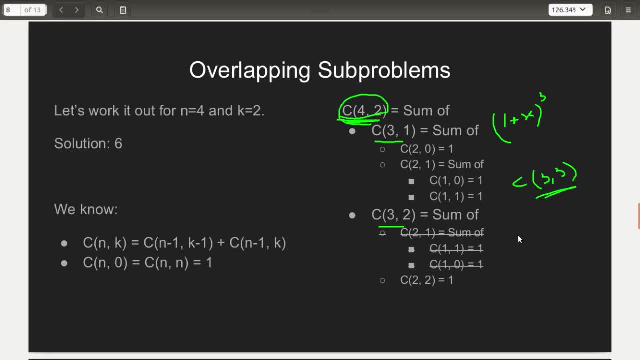 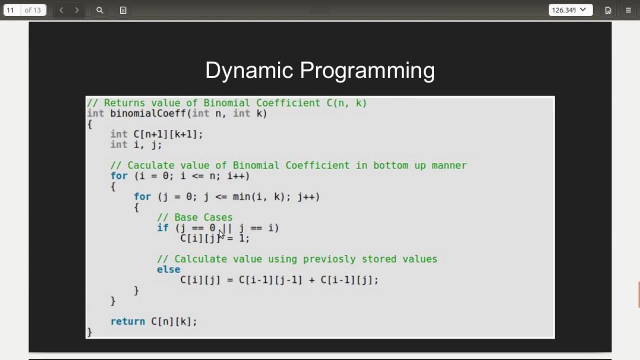 three or any such computation where, let's say, for different values we will need to have values of n. we won't need to calculate any value of n, c, k where k is actually greater than two. so this is why we have that condition in our looper here, min i comma k, and so that 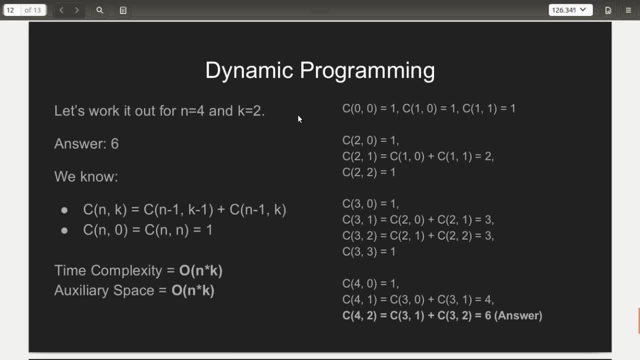 so let's let's look at how this code works for the same example, as we saw earlier. so for n is equal to four and k is equal to two. let us look at the dry run happening over here. so for i is equal to zero, we calculate this value. and for i is equal to one, we calculate. 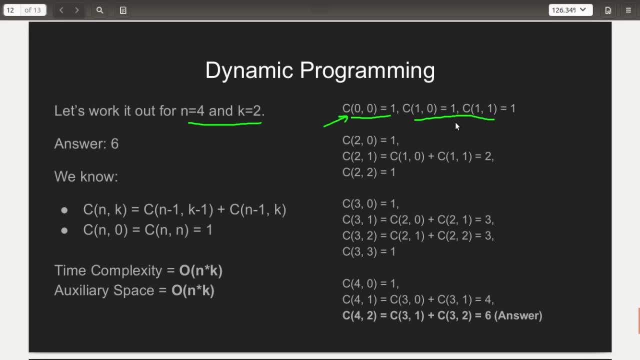 these values. now, these all these values satisfy the base conditions. so we simply put in one whenever we wanted to calculate these values, and for i is equal to two- we calculated these values. now we see over here, when we were calculating c, two comma one, we needed to have the values. 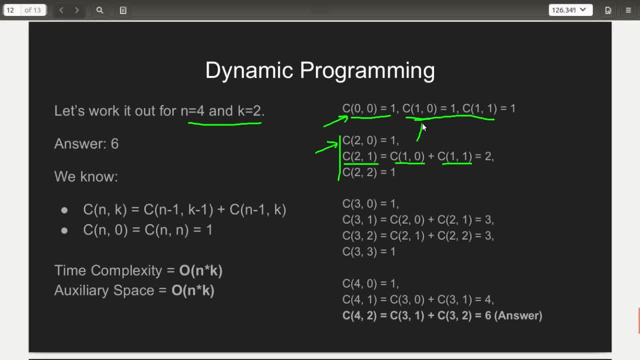 of c, one comma zero and one comma one, and we had already computed these values. so this time we did not solve these problems again. instead, we just did a lookup. and that same thing is again repeated over here. instead of solving the same problems again, we simply did a lookup.